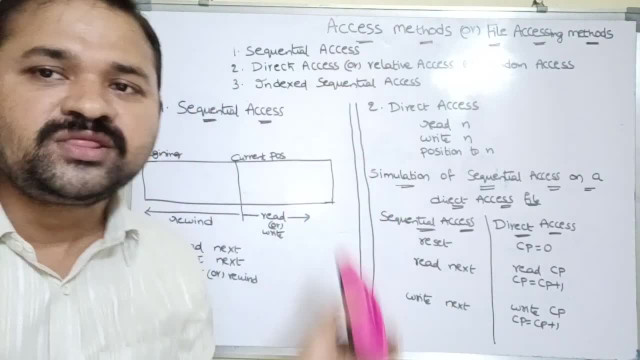 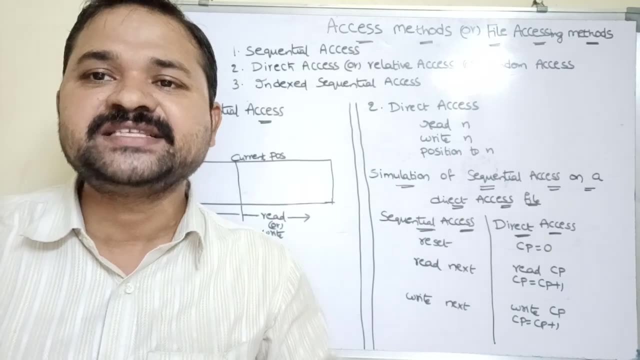 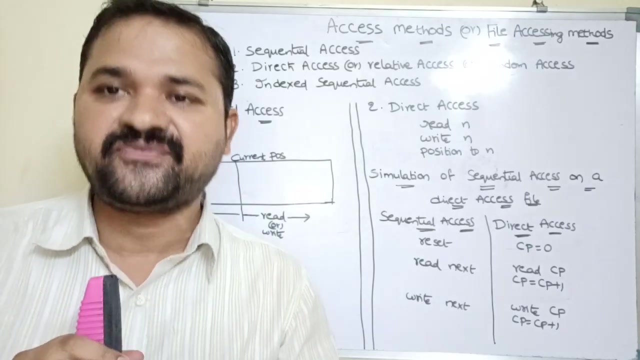 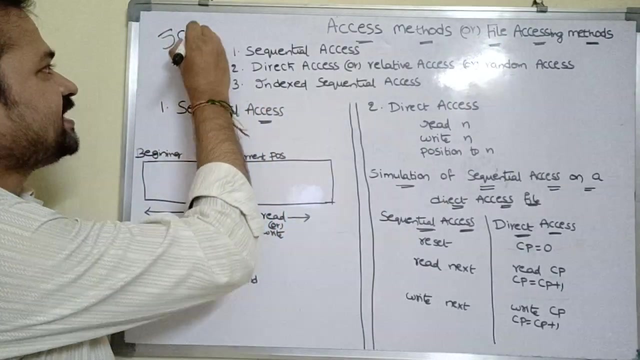 Sequential access is the simplest method of all the three methods. Here the name itself specifies the meaning. The information in the file is accessed in sequential manner, that is, record by record. Let us assume that we have a file which contains 100 records. Let us assume that currently we are at 50th record and we want to access 75th record. 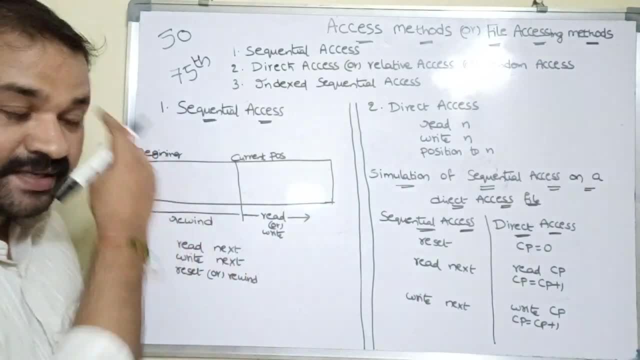 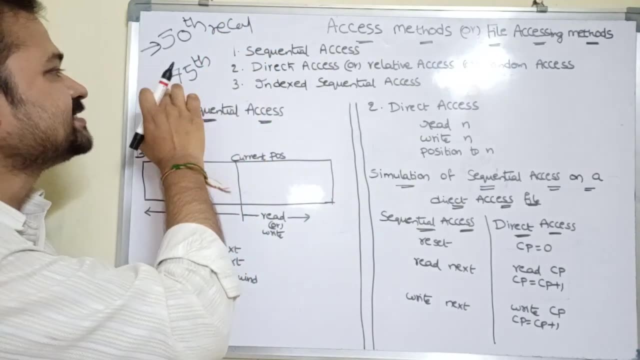 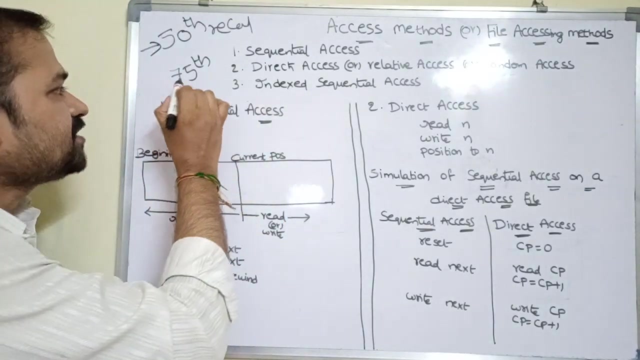 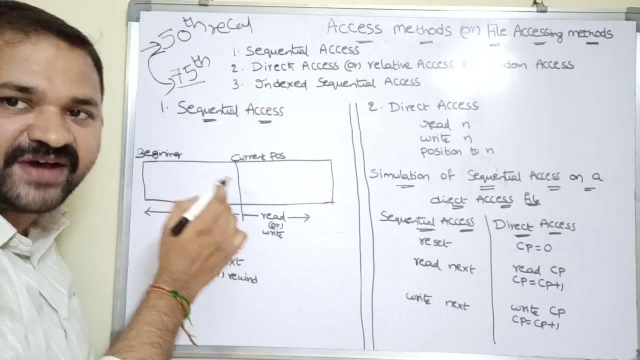 But which accessing technique? we are using sequential access. So in order to access 75th record, we need to access all the records from 50 to 75. So first we need to access 50,, next to 51,, next to 52,, 53, like that. 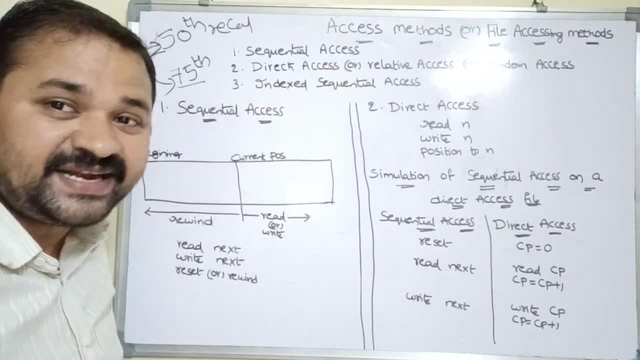 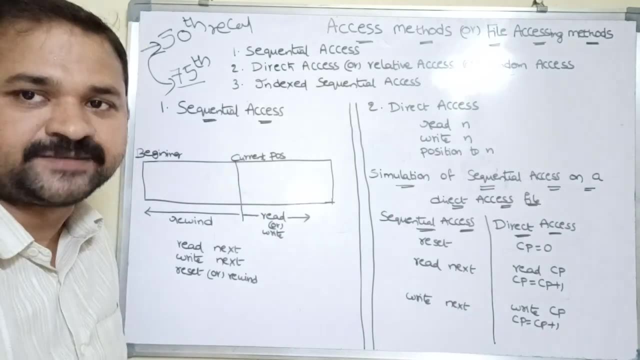 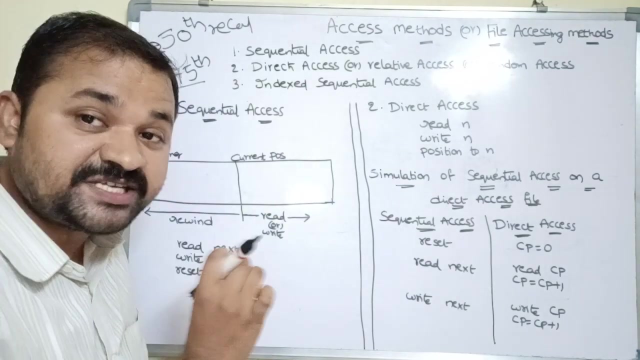 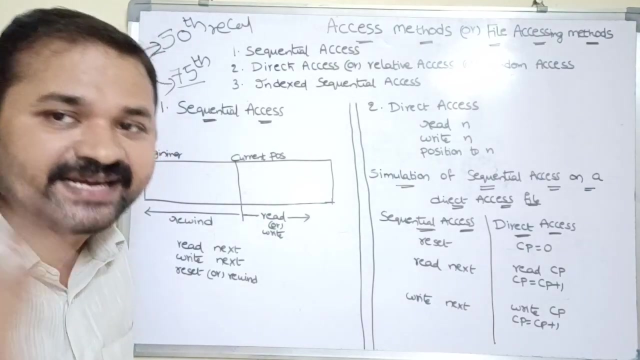 So it is not possible to access 75th record directly. So all the records in between 50 to 75th are to be accessed. Why? because sequential access means all the records are accessed in sequential manner. So what is the problem here? It will take more amount of time in order to read that record, in order to access that record. Why? because we need to access the records between 50 to 75 also. 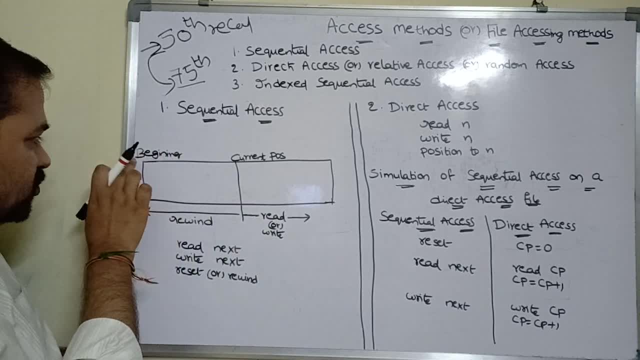 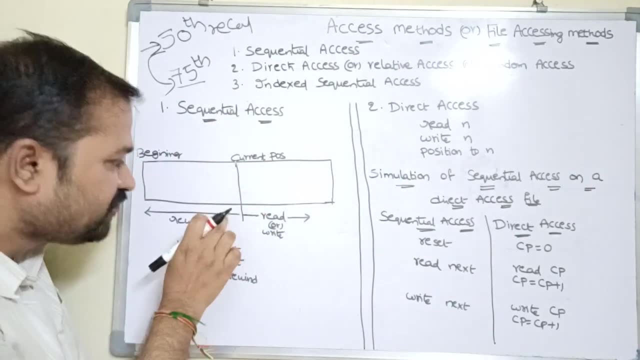 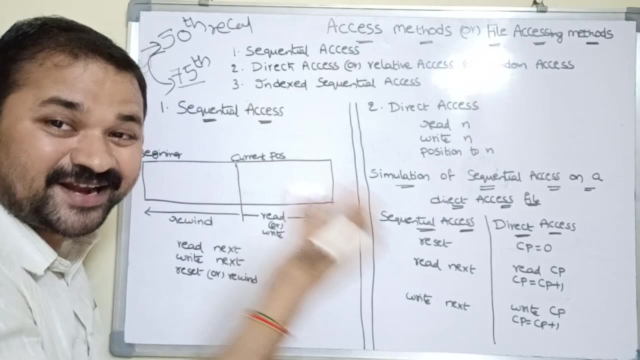 Let us take the diagram here. So this is nothing but beginning of the file. So this is nothing but our current position, head. So let us assume that now we are yet at this position. So after that we have to perform either read operation or write operation, record by record. 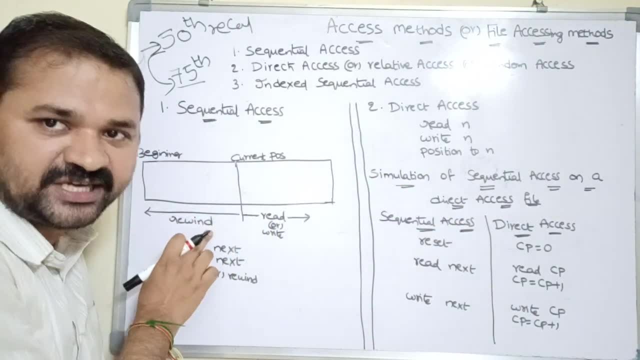 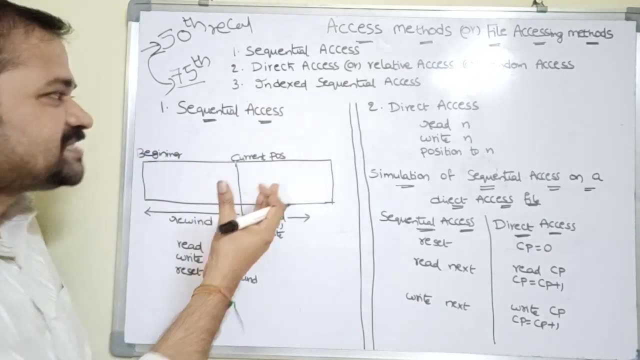 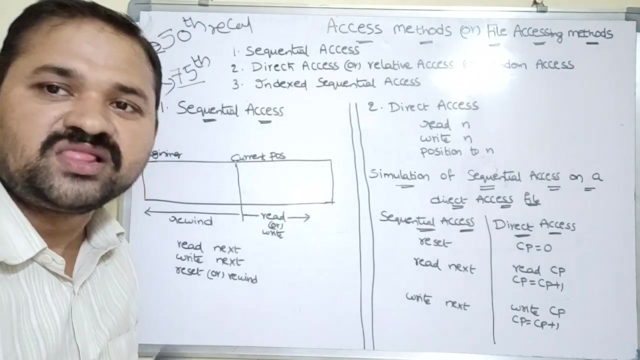 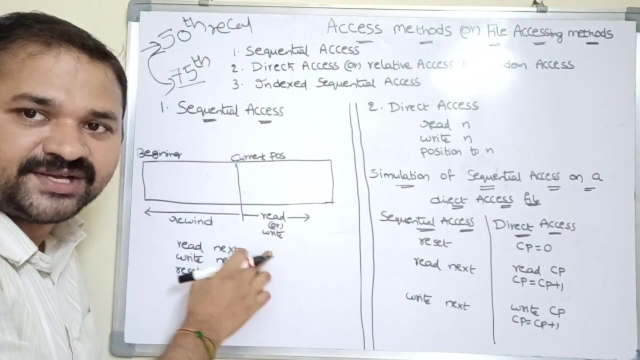 Next, if you want, we can perform the rewind operation. Rewind means reset operation, So that means moving to the beginning position of the file. What we are seeing here is the tape recording, So at the beginning of the file we are following the爓ạ. 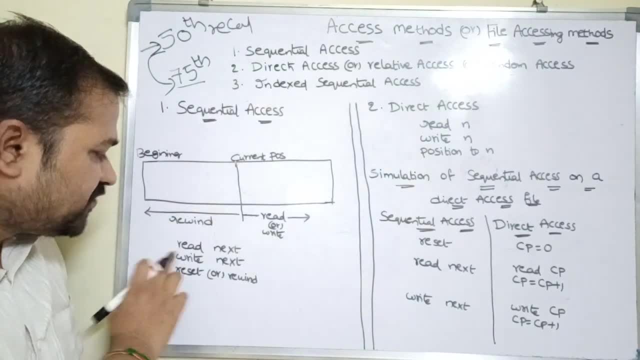 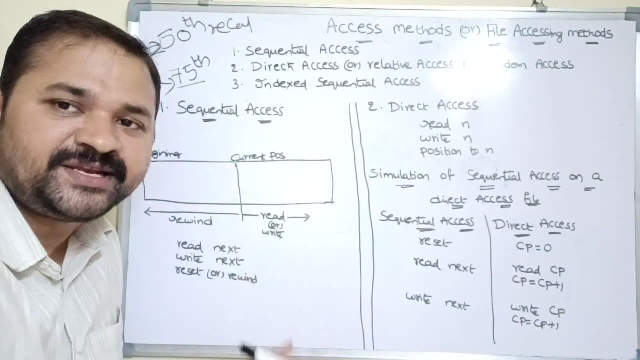 seemed required information. The level of the record depends on what you are using: your phone, of course. As it is the fourth generation, there will be an extra video reference. and, of course, record is time iest one And remember when you sleep near your bed. it will be agenda when you go to bed, surely? 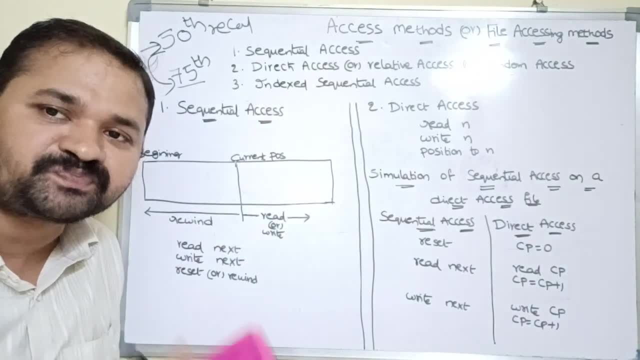 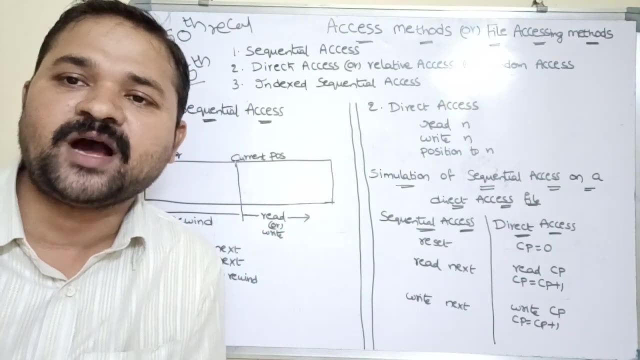 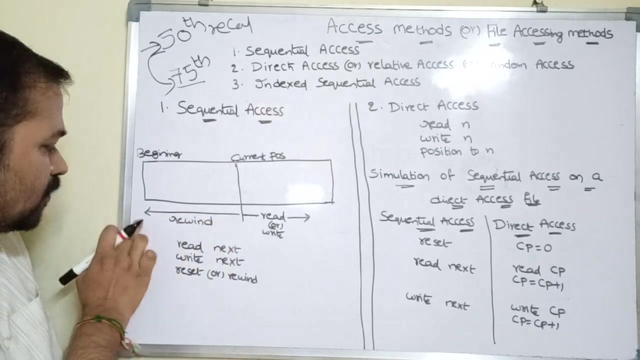 position likewise after writing the next record also. uh, then the right pointer will be moved to the next position. that means the read pointer as well as the right pointer will be updated while performing readness and write next. next one is reset or rewind. so reset or rewind means 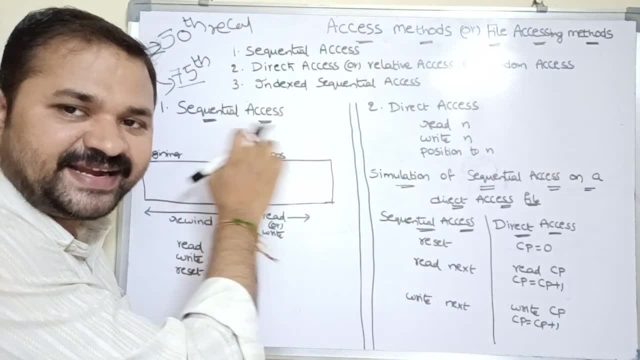 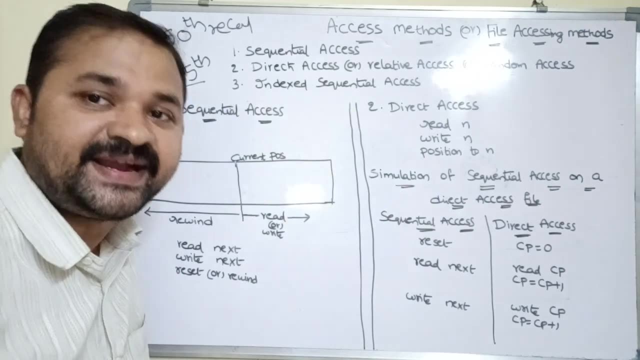 moving to the beginning position of the file. so the major advantage of this approach is it is the simplest technique. we have to access all the records one by one. but the major disadvantage is it is not possible to access any record directly. that means it will take small amount. 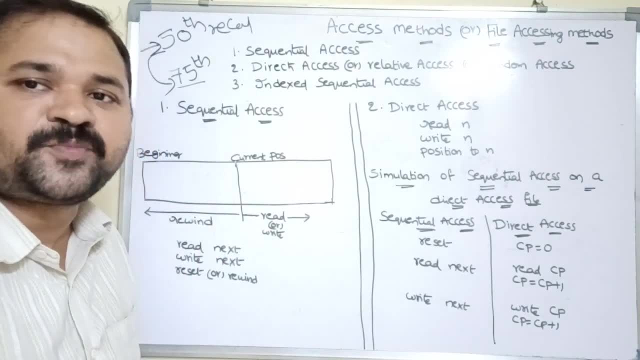 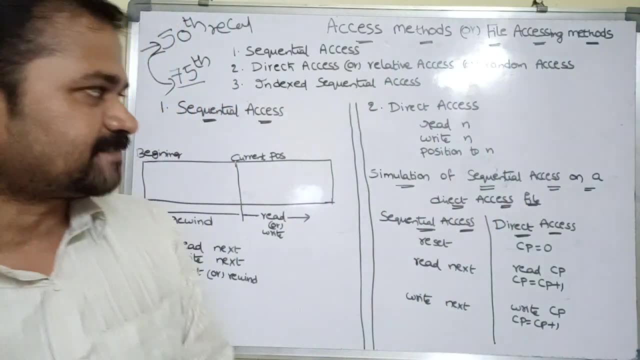 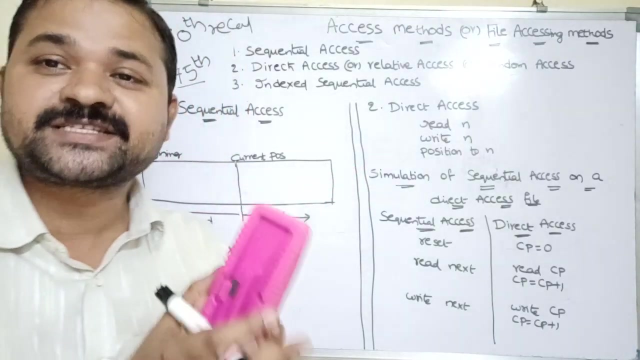 of time in order to access that record. so we can overcome the problem with the help of the second technique. so the second technique is direct access, or relative axis, or random axis. so by using this technique we can access any record directly. let us assume that our file contains 100 records. 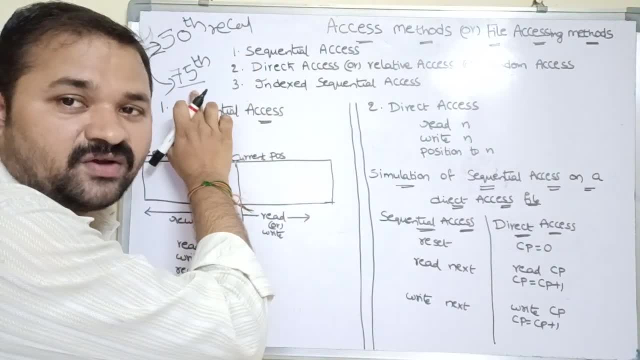 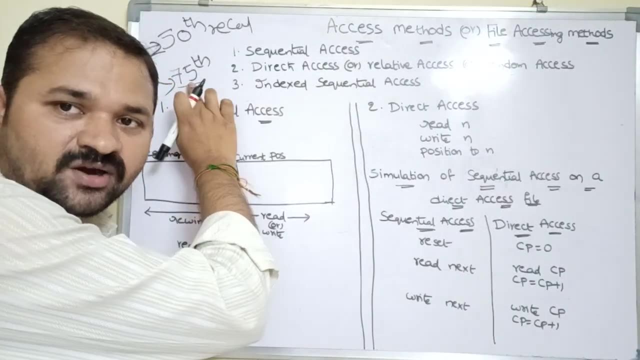 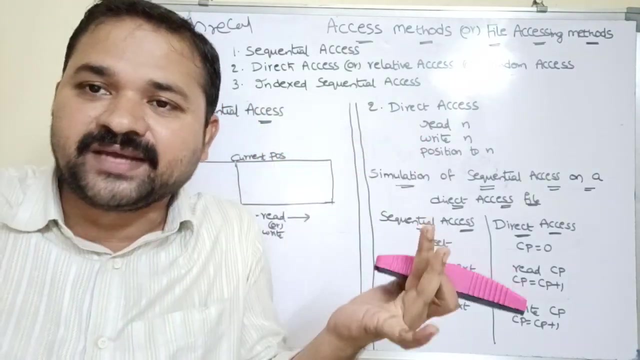 like. currently we are at 50th record and our target is we need to access 75 record. then directly from 50th record to, we can go to the 75th record as well as we can access the 75th record. so that is the advantage here: we can access the record randomly without worrying. 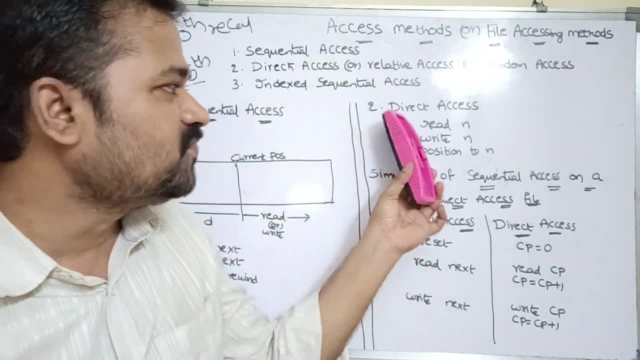 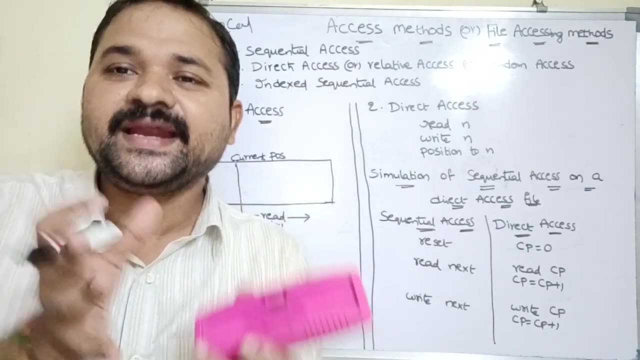 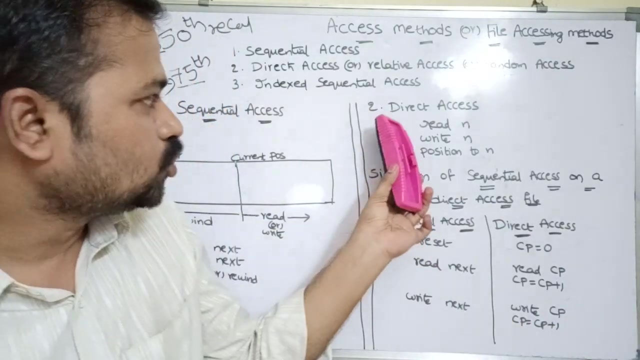 about what is the order. okay, so the best example for direct access is hot disk, magnetic disk. so we know what is a magnetic. a magnetic disk is it is organized into a collection of blocks where the blocks contains the files. okay, so the best example here is: if you take a CD, let us assume that CD. 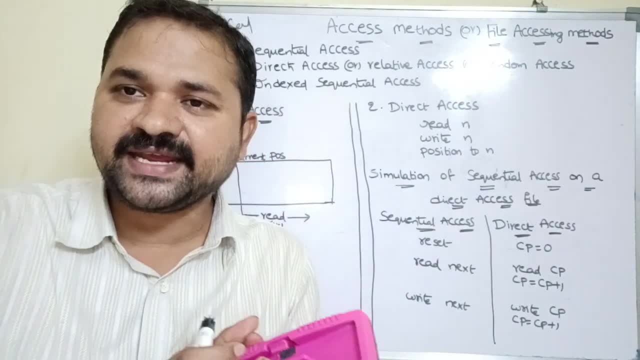 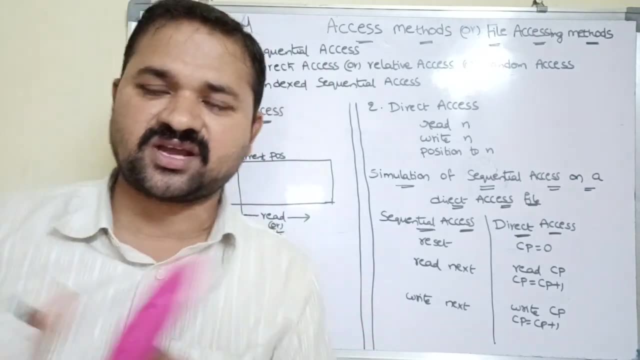 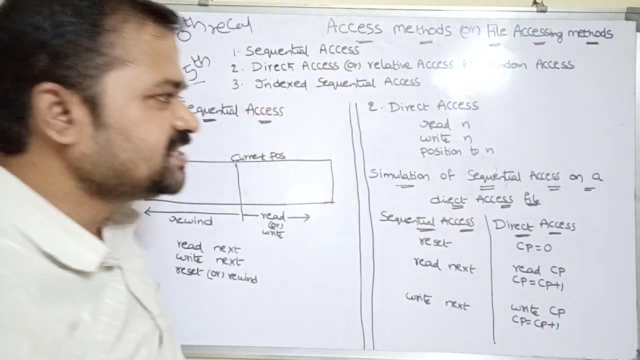 contains 10 songs and it is assumed that now we are yet the third song, so we are listening the third song, then directly we can go to either seventh song or ninth song or tenth song. so magnetic disk, such as CD, hot disk, so these are the best examples for direct access. okay, let's see the 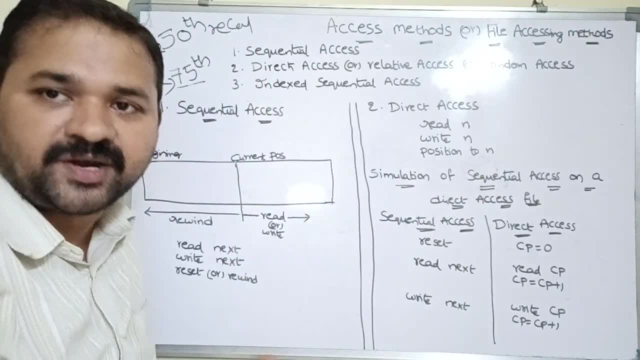 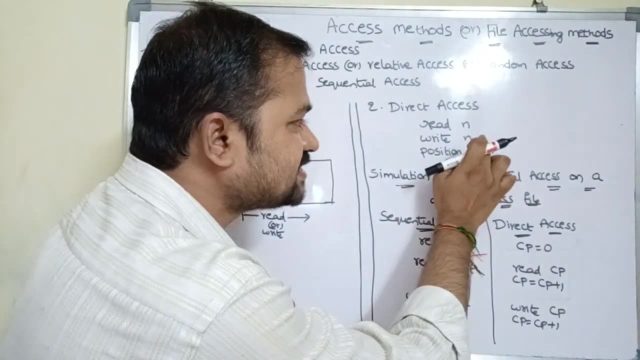 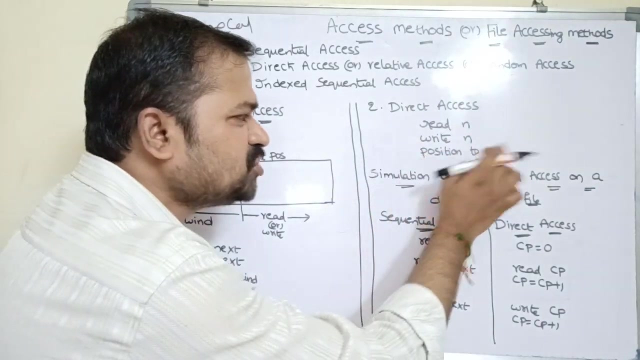 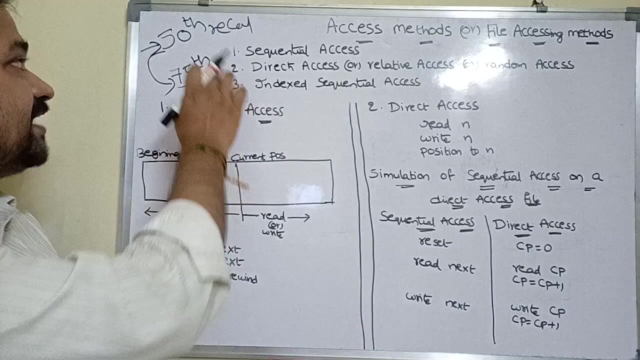 operations: here read n. here n means block number. okay, so read the fifth block number, seventh block number, ninth block number, tenth block number, like that. okay. next one is write n, so write the content into the block number. write the content into n. next one is position to n, so we can move the position at at any block as we want. so let us assume that now we 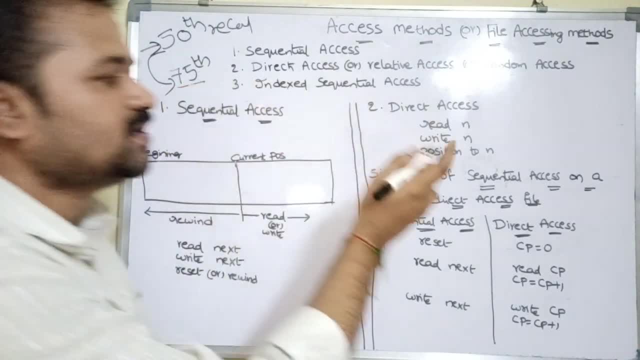 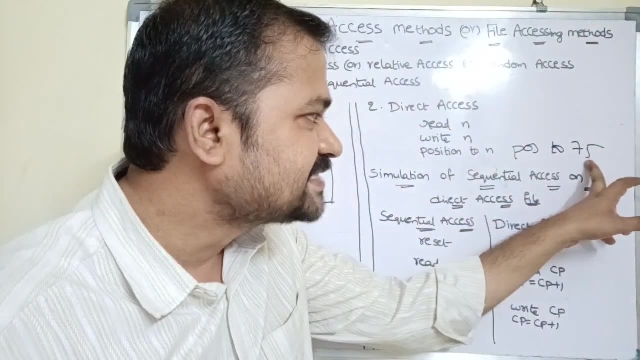 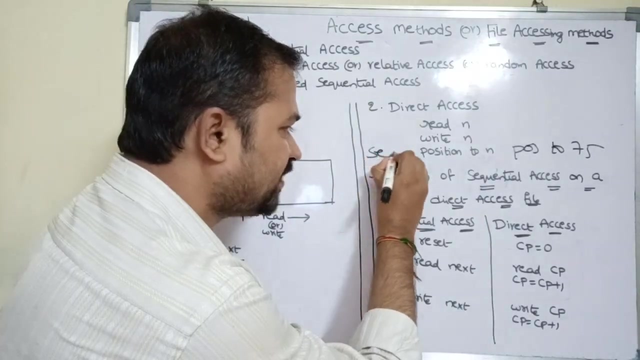 are at 50th block and we want to move to the 75th block, then we can write as a position to 75. so let's say 75th block, okay. so after that we can perform either read operation or write operation. so position is nothing but the seek operation that we use, as in the C language. this position 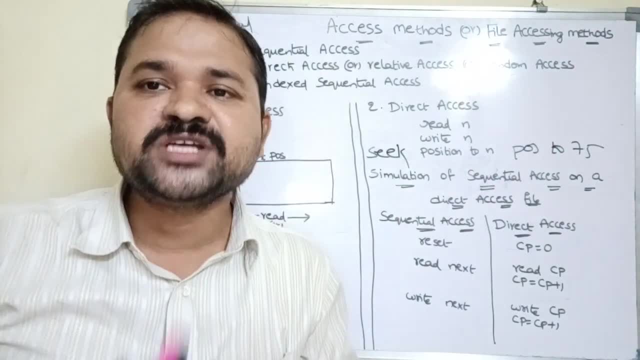 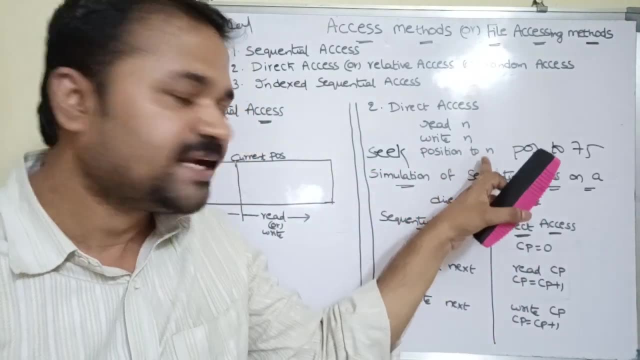 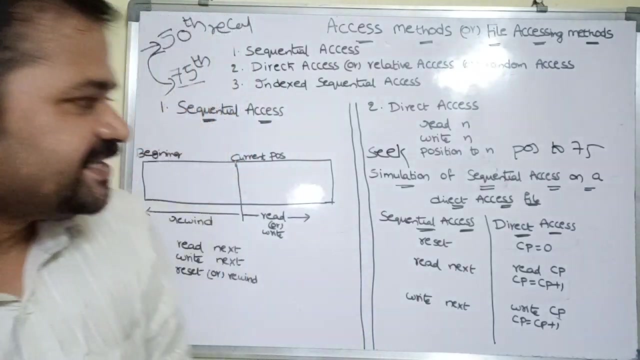 doesn't involve any input and output operation. by using position we can place the file pointer, yet any position as we want here. position means read operation doesn't involve write operation doesn't involve only we are moving the file pointer to the specific block. now let's see the simulation. 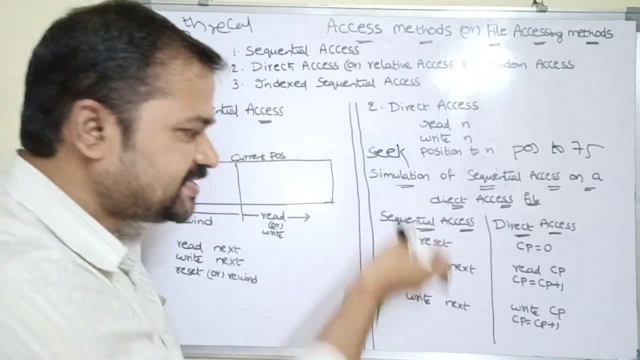 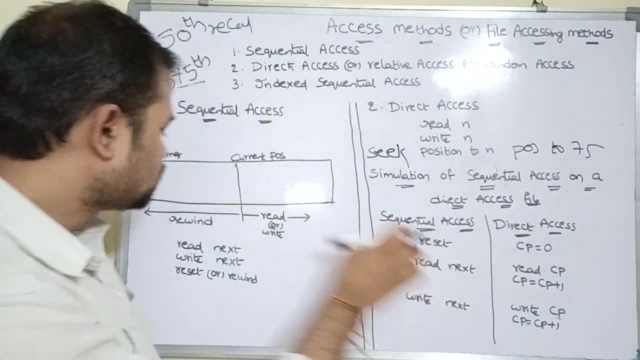 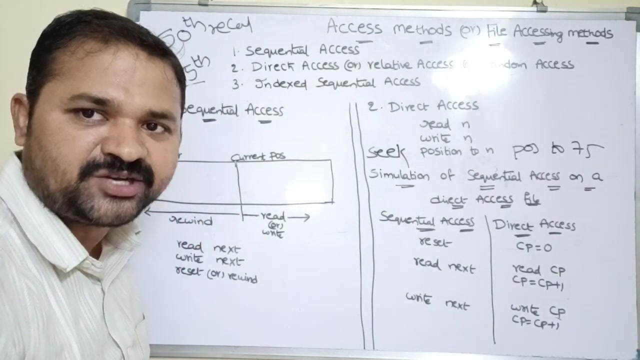 of sequential access on a direct access file. so this is nothing but sequential access. this column is nothing but direct access in sequential access. like we have a command like reset, so reset means moving the position- current position- to the beginning of the file, so moving the file pointer. 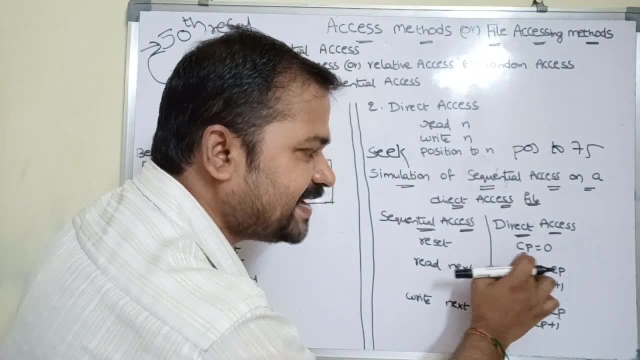 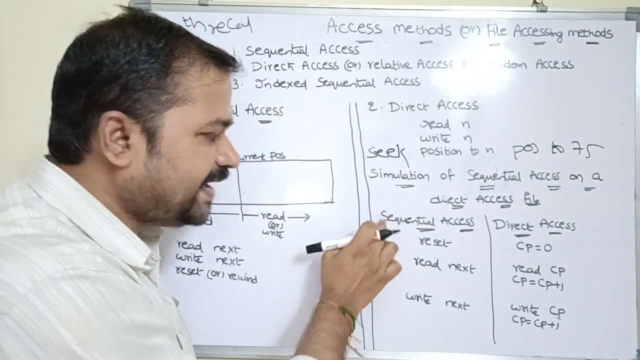 to the beginning of the file various indirect access. we can write here: CP is equal to zero, current position is equal to zero, so that CP will be placed at the beginning of the file in sequential access. if the statement is like this, read next. so if you just read next, then what will happen? the 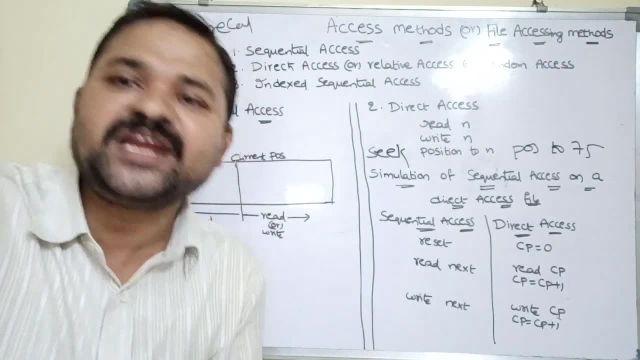 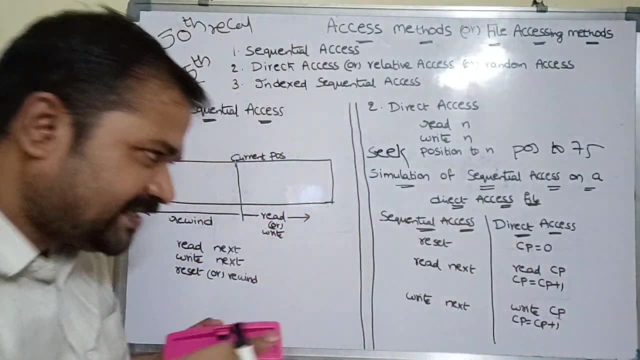 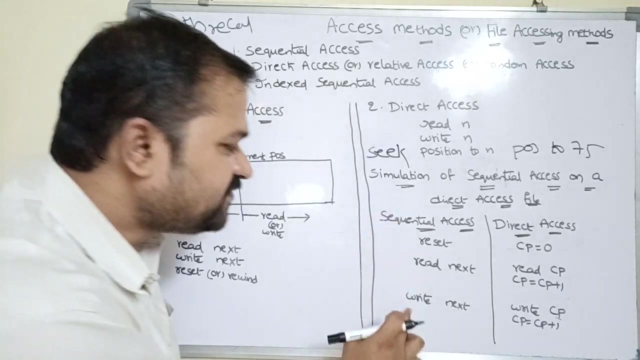 corresponding record will be read it and after that read pointer will be advanced to the next position. various indirect access. we can write as read CP. so read that value. then after that, CP is equal to CP plus one, so that the current position will be moved to the next position in sequential. 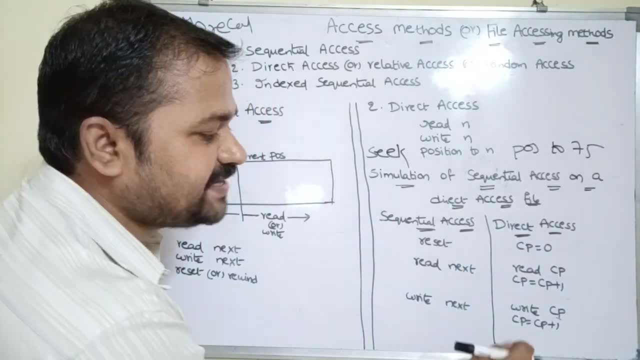 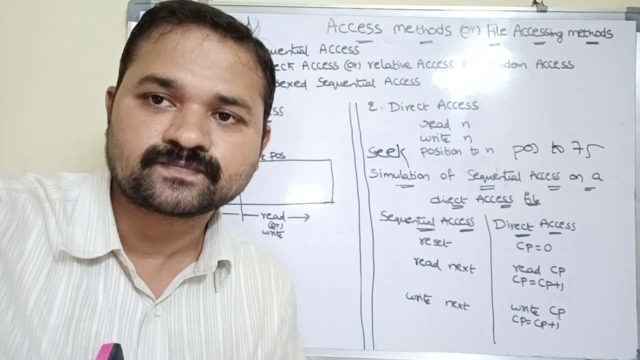 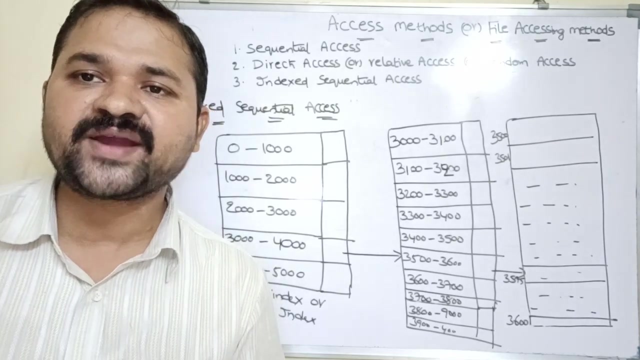 access. if the statement is like this, right next, indirect access. we can write as write CP and after that delete. so this is about direct access. now let's see about indexed sequential access. it is mainly useful in order to overcome the drawback of sequential access. we know that the major drawback 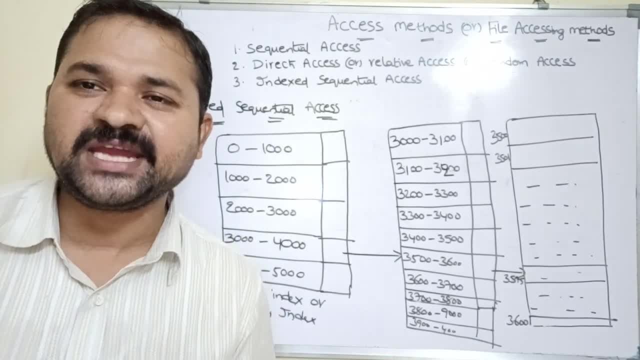 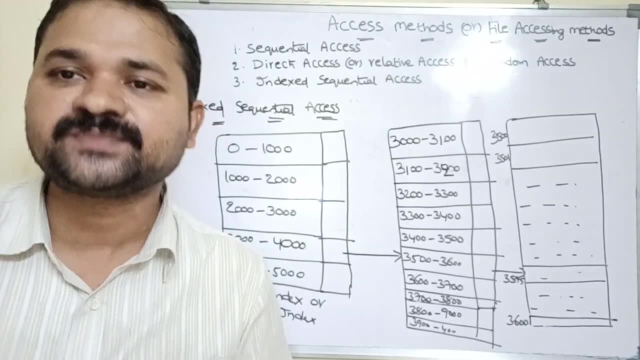 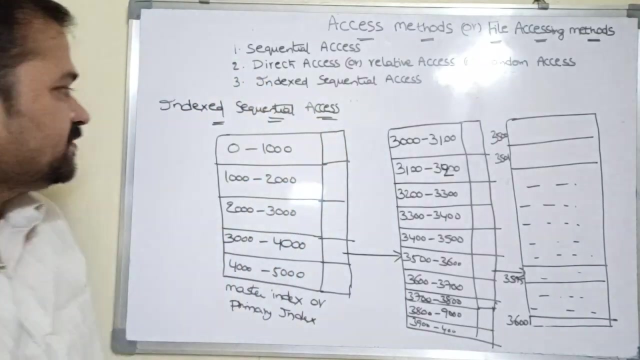 of sequential access is for accessing a record. it will take more amount of time. why? because in sequential access all the records are processed or accessed in sequential banner. okay, uh, indexed in axis. the name itself specifies the meaning. here. it works based upon index. okay, let us assume that. 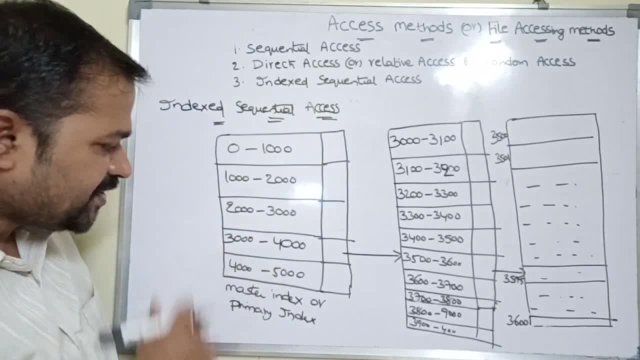 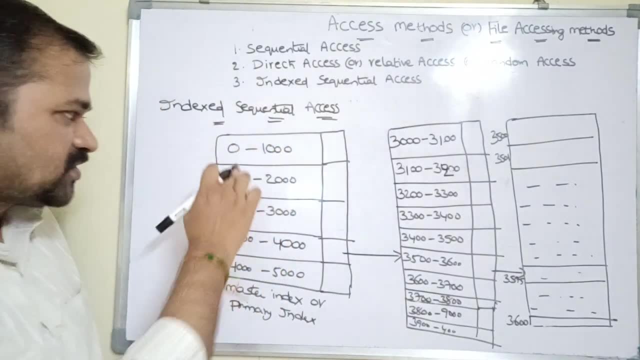 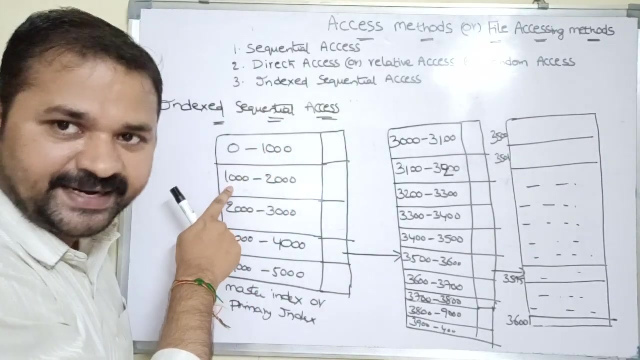 we have a 5000 records. then the 5000 records can be divided into six blocks where each block contains 1000 records. so the first: here we have 5000 records. the first block contains the records from 0 to 1000. second block contains the records from 1000 to 2000. so likewise, each block contains: 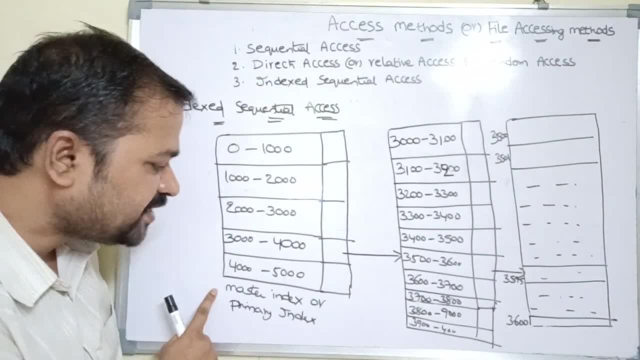 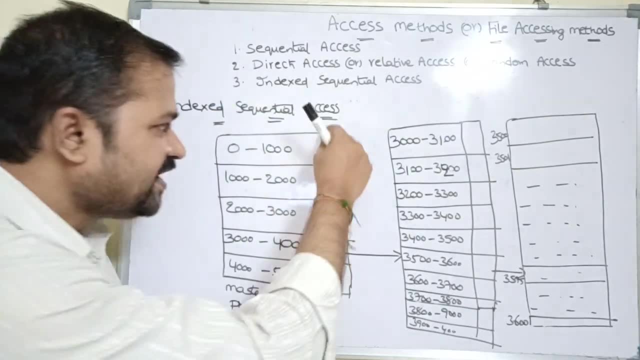 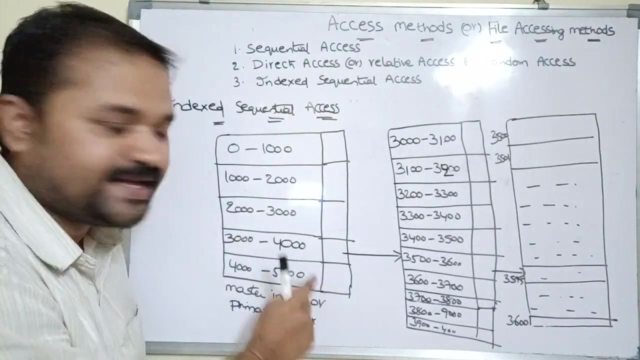 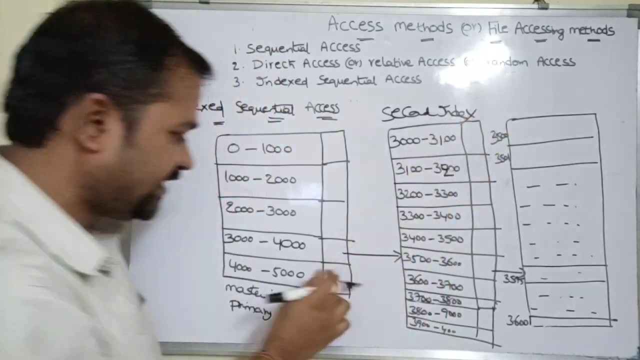 thousand records, so this is known as master index or primary index. so it contains two columns. the first column is nothing but records, whereas the second column is nothing but pointer. so master index or primary index contains a pointer which contains the address of secondary index, so this is known as the secondary index. okay, so here we have a pointer, so this pointer. 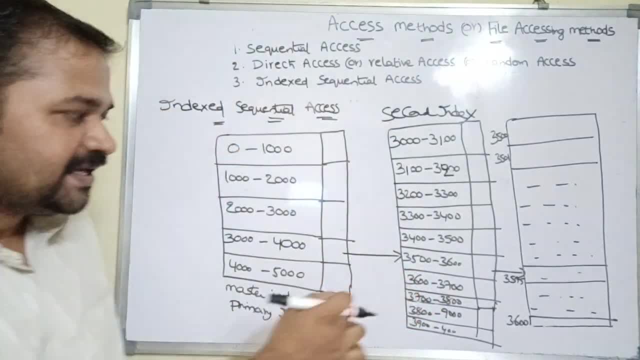 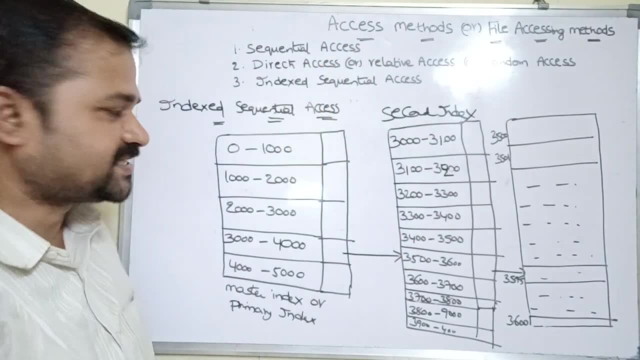 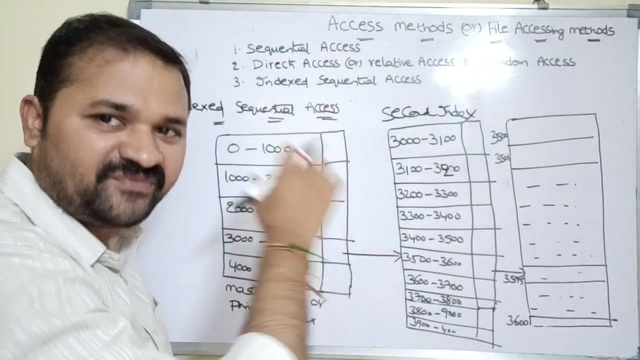 contains address of the second, one secondary index. so this secondary index. let us assume that here for each block we can have a separate secondary index. so from 0 to 2000 we can have a separate secondary index. from thousand to two thousand we can have a separate secondary index language. here we have drawn the secondary 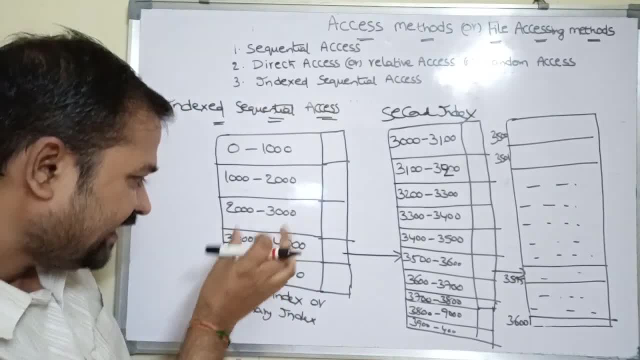 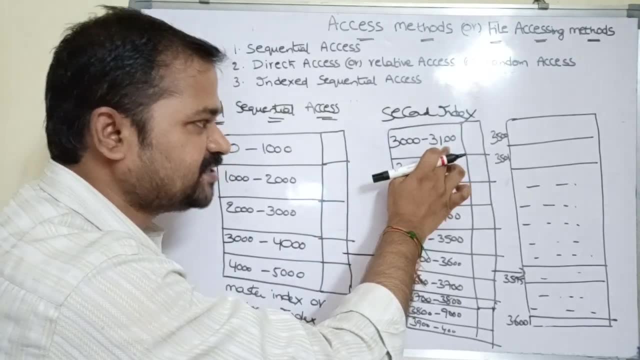 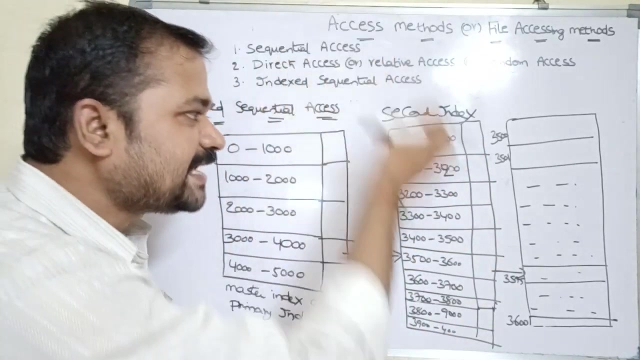 index for three thousand to the four thousand. so we can divide these thousand records into ten blocks where each block contains hundred records, so from thousand two to three thousand one. so this is nothing but first block. three thousand one hundred to three thousand two hundred, so this is nothing but second block. in secondary index also we have two columns. so the first column 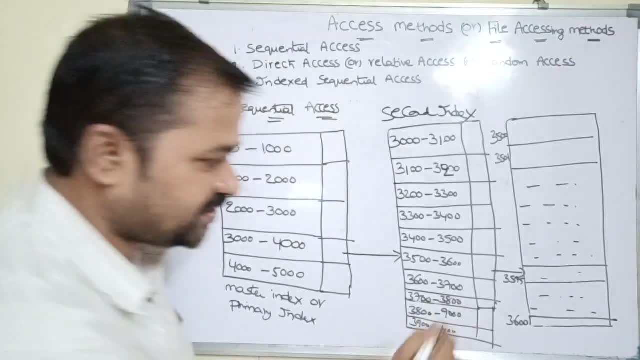 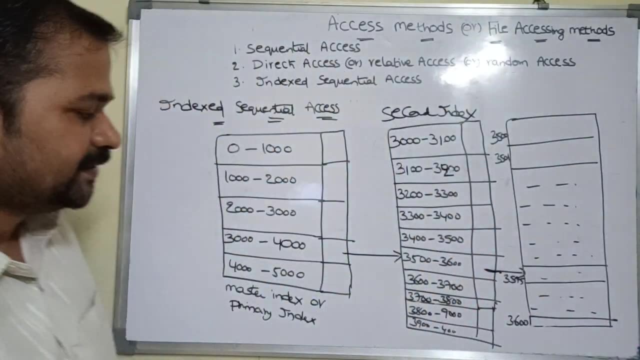 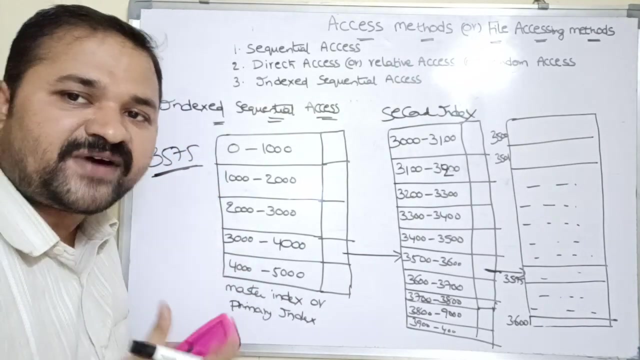 specifies records, whereas the second column specifies the pointer. so secondary index pointer contains the actual data of the corresponding record. okay, in this example, let us assume that we want to access record. so first here, in order to find this record, we can apply binary search on this algorithm. so 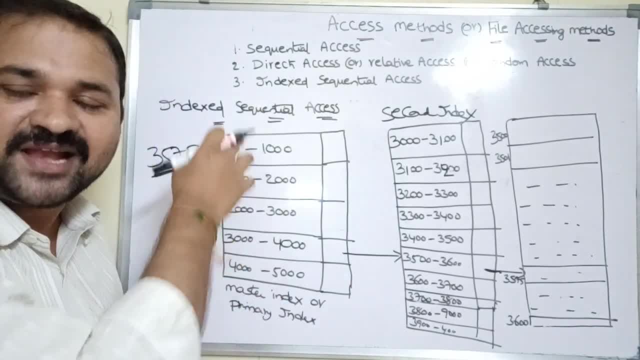 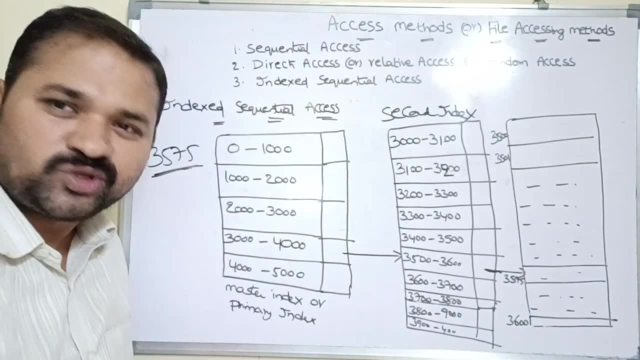 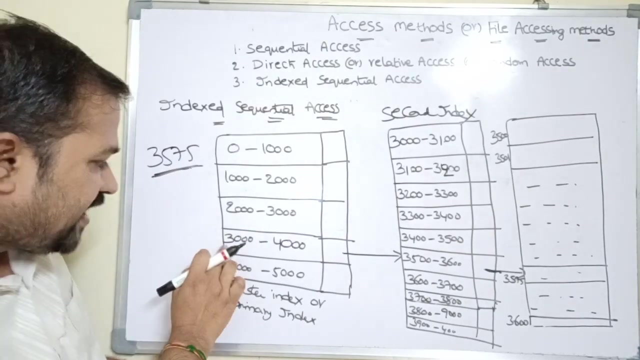 that the number of comparisons will be less. we have to calculate mid value. mid is equal to low plus i by two. so compare 3575 with this zero as well as this 500, so that the number of comparisons will be less. okay, if we apply the binary search on this master index. so here we have three thousand.